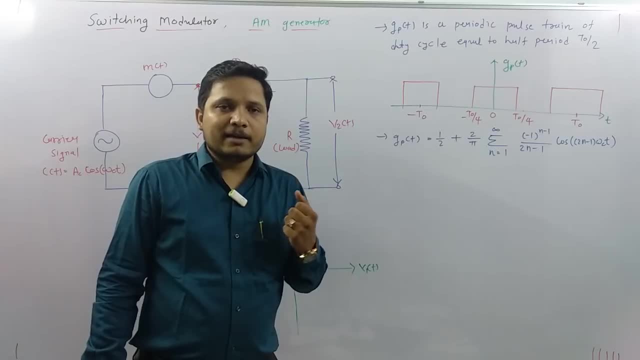 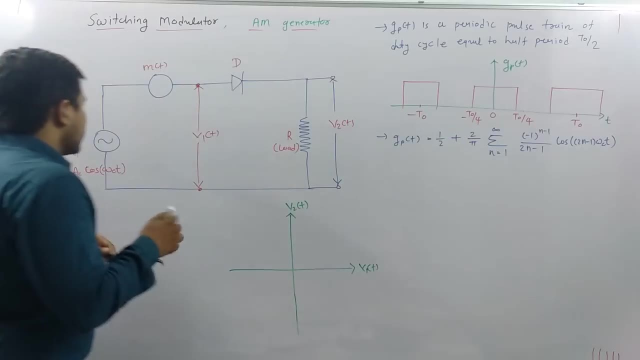 So let us see, step by step, what are the things which is happening inside, and then at the end, you will be able to understand how AM signal is getting generated. So here, carrier signal that is connected in series with modulating signal. So, as it is connected in modulating signal resultant of these two series, that will be 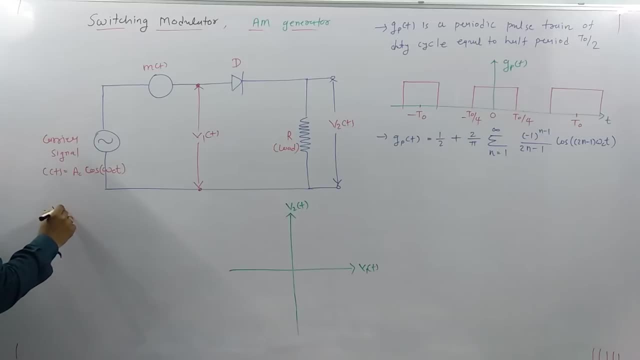 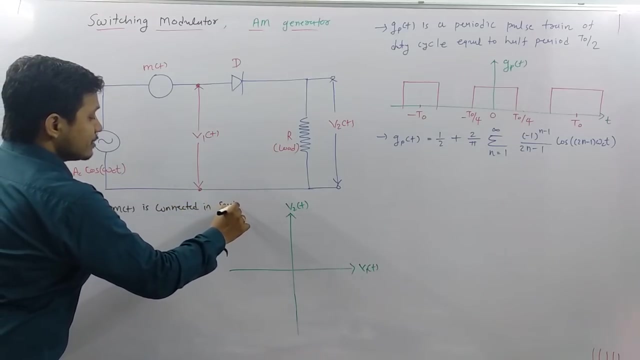 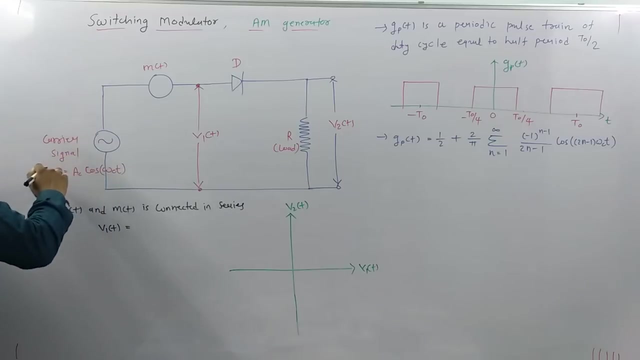 V1T. So CT means carrier signal and MT means modulating signal is connected in series. So we can say V1T, that is carrier signal, MT plus CT. where CT is AC, cos, omega T, You can consider even carrier signal as a sign. there is no issue with that. 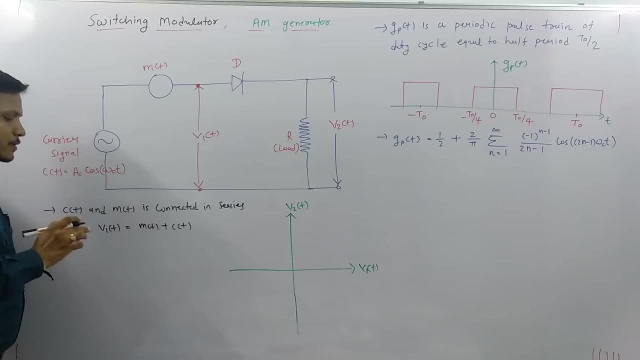 Here I have considered it as AC cos omega T, So this V1T, that will be MT plus AC cos omega CT. Now see This V1 signal now that is passing through this diode. And one more thing that we need to understand when this is what connected in series value. 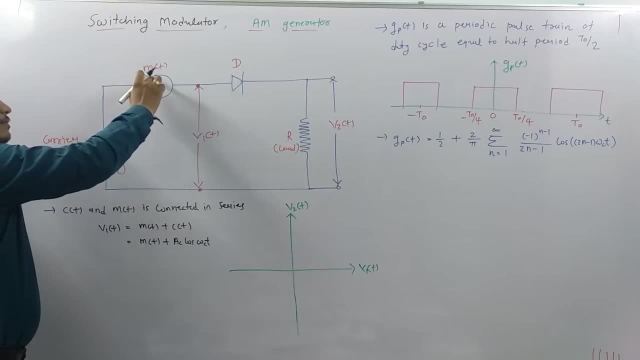 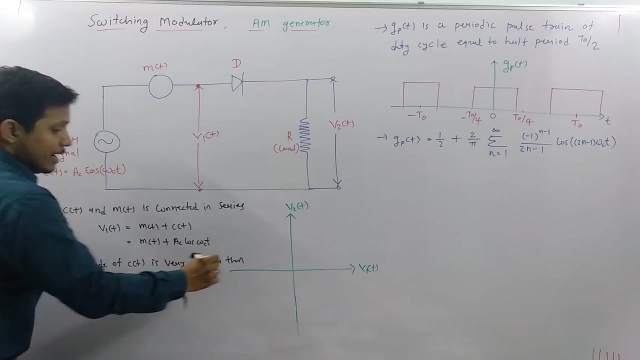 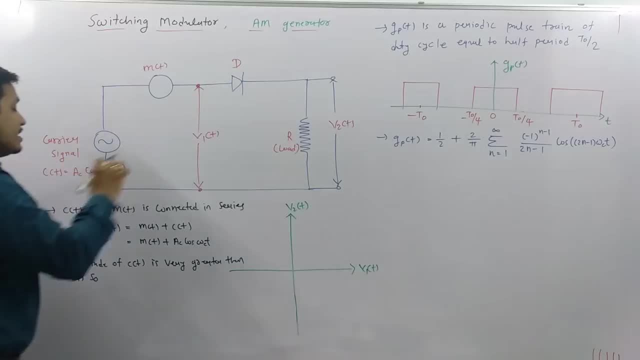 So is died on and off. That is being justified by carrier signal. The reason is amplitude of carrier signal is very greater than amplitude of modulating signal. So on and off, That will get justified by carrier. No little change by carrier signal. I will show you that, how it is turning on that diode and 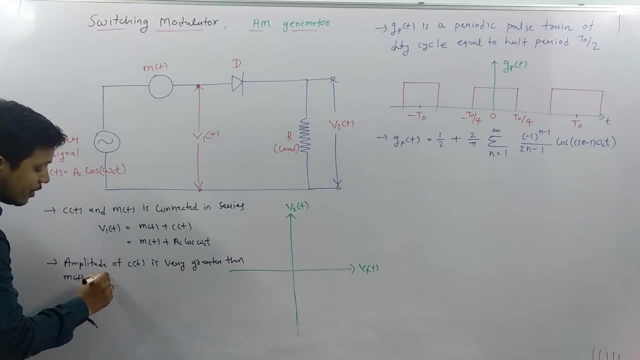 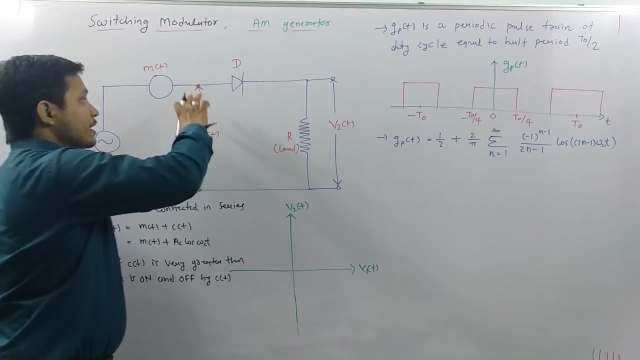 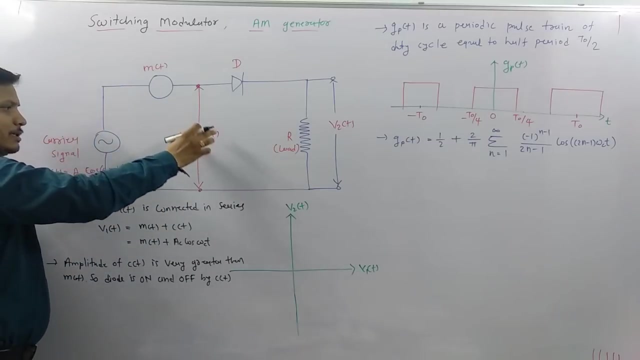 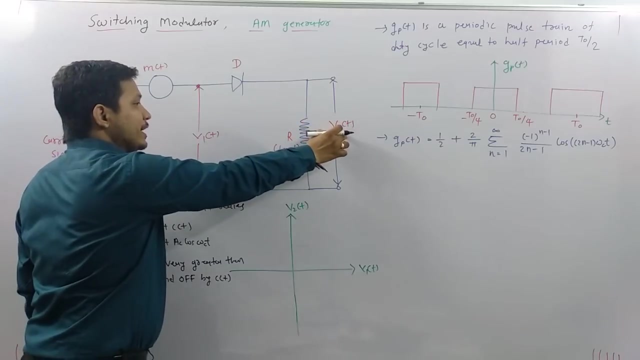 turning off that diode. so diode is on and off by CT only. so ultimately you will be observing if this carrier signal that is greater than this V1t. so in that case this diode is on and you will be getting output V2t, that is equals to V1t. so 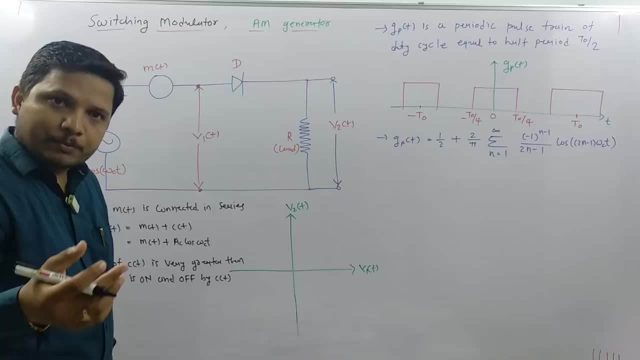 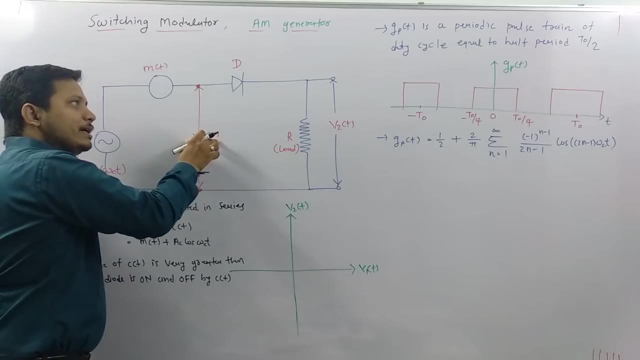 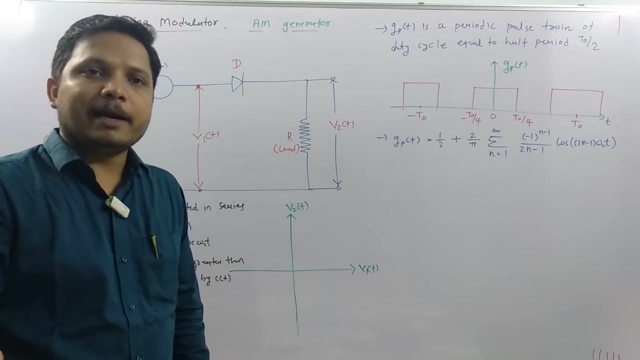 if carrier signal, if I say it is positive, in that case this diode will come in forward bias and whatever V1t that is there which will be getting transferred at load side. so there are two cases that you need to understand. one is whether CT is positive and second is whether the CT is negative. so if 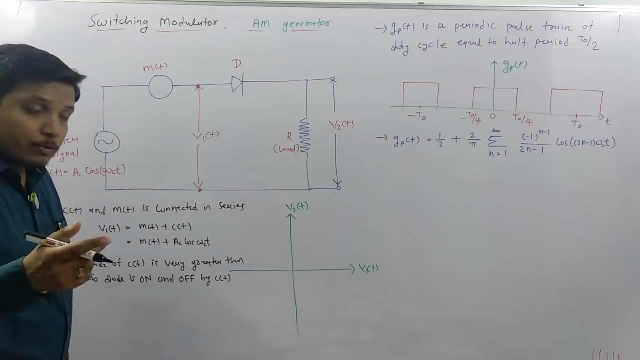 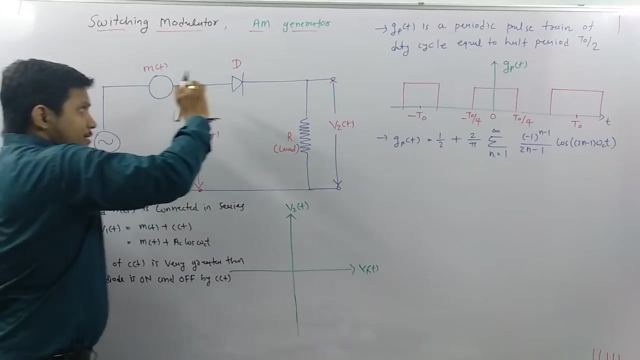 this carrier signal. if it is positive, then this V1t that will get transferred over here because of diode is getting on, And if CT is negative, in that case this diode will be off. So output V2T that will be zero. So if we see the graph in between V1T and V2T then it is purely 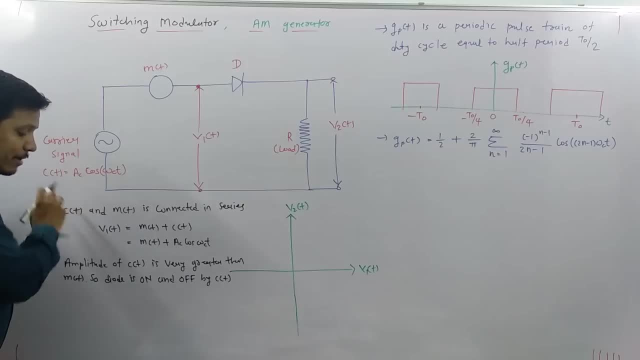 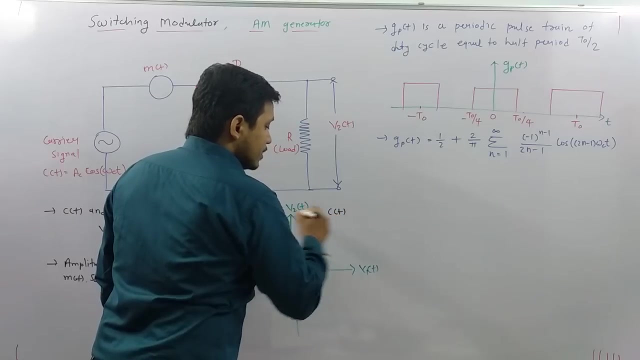 based on carrier signal amplitude. Why? The reason is: carrier signal amplitude is very greater than modulating signal, So diode will turn on and turn off by carrier signal amplitude. So there are two cases. First is CT is positive. So if CT is positive means 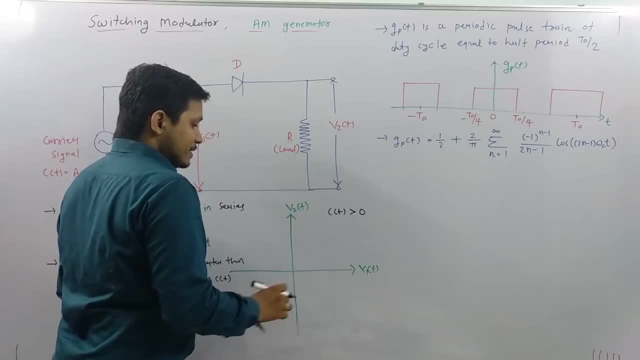 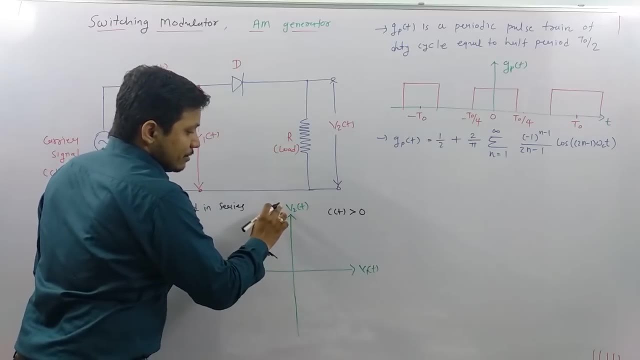 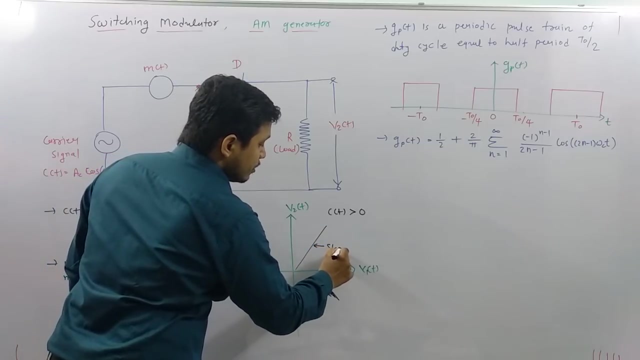 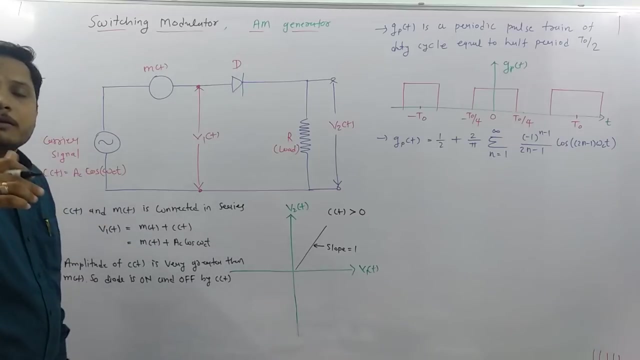 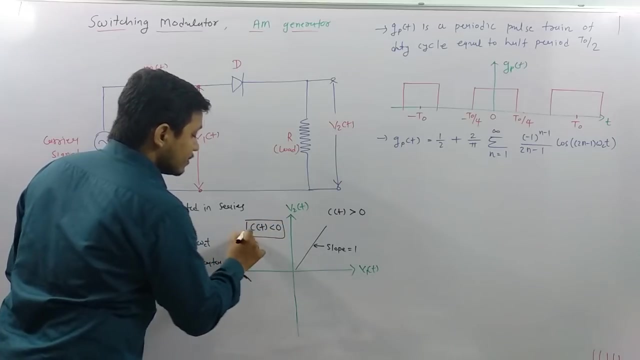 CT is greater than zero. So if CT is greater than zero, V1T that will come over here. So ultimately, graph in between V1T and V2T- that will be straight line with slope- is equals to one. But if CT that is having negative value means if CT that is less than zero. So if CT is, 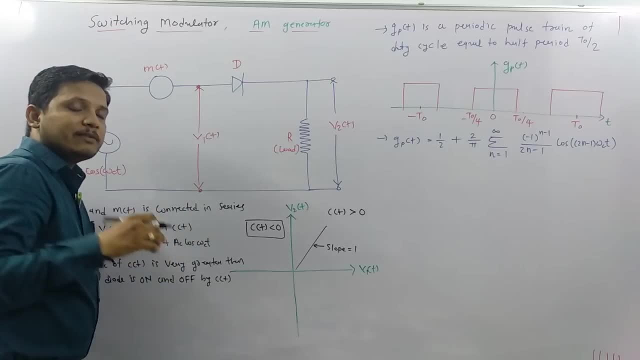 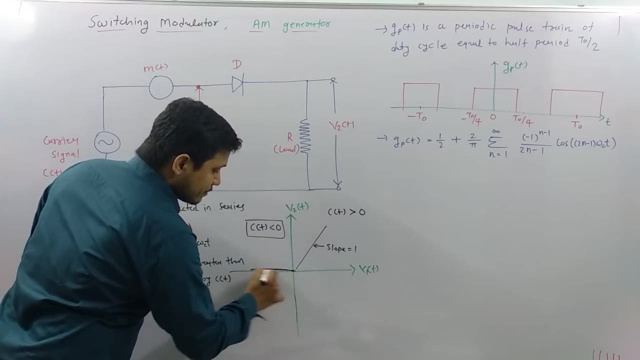 less than zero diode will be off. And if diode is off, output V2T will turn off. So output V2T will be zero. So you will be finding line is like this: So ultimately V2T output. 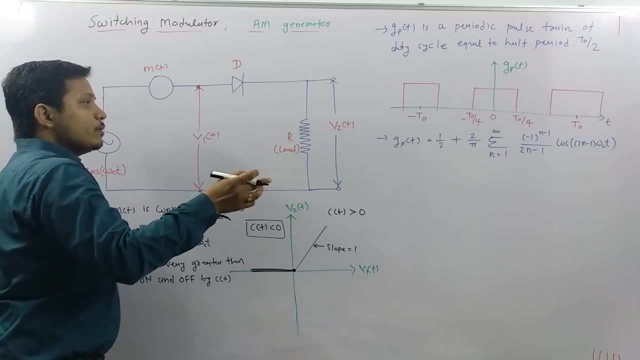 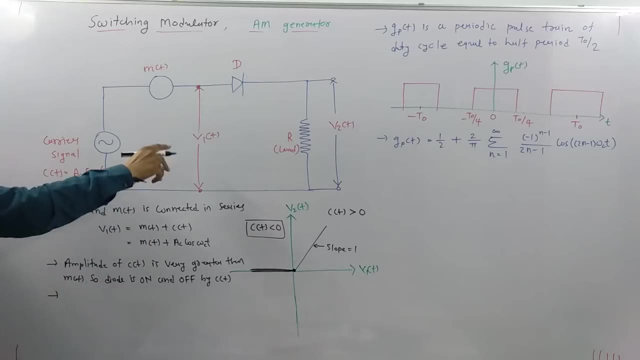 that is varying in between zero and V2,, V1T. So here one can say output V2T, that is V1T, Where CT is positive means greater than zero. So output V2T will be 0. So you will be finding. 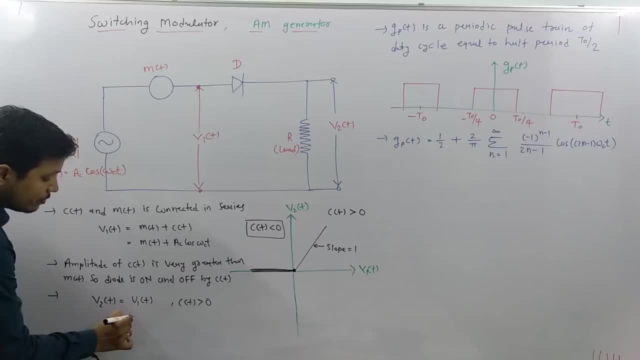 line is like this: So, ultimately, output, V2T output that is varying in between zero and V2T- is greater than zero, And V2T output that will be zero in case of CT is negative. It means it is zero. So that is how things are happening. Now see one thing that is: 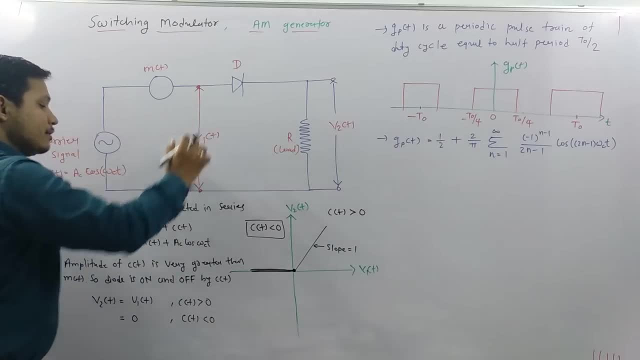 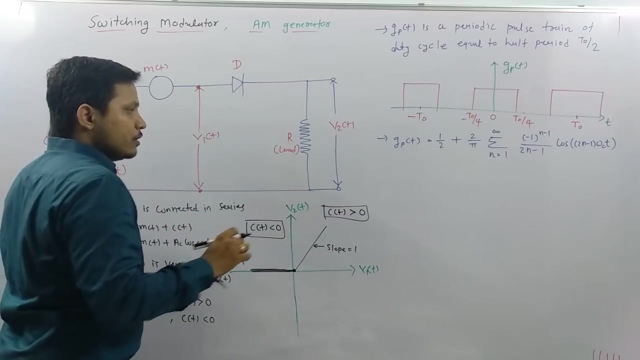 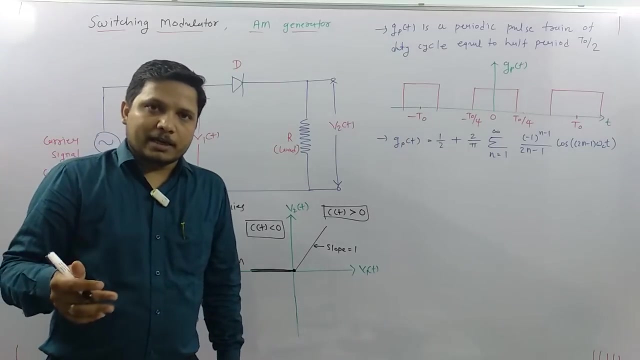 very clear to all, like how this diode is turning on based on value of carrier signal. If it is positive, then this V1T that will go to output And if this value of CT that is negative, output will be zero. So V2T that is varying in between V1T and zero periodically, So with 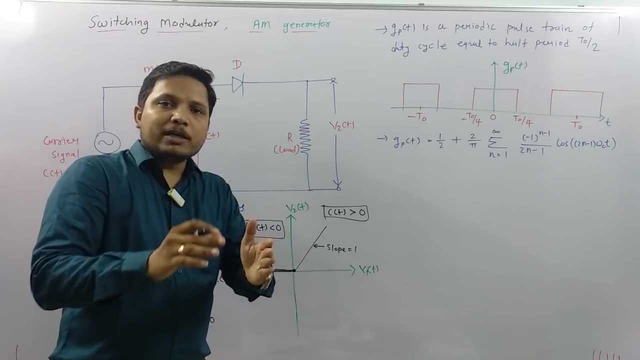 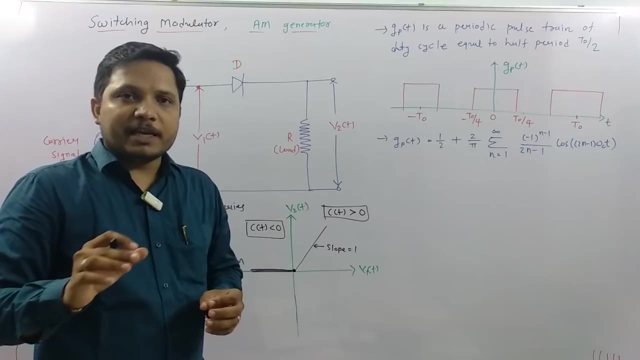 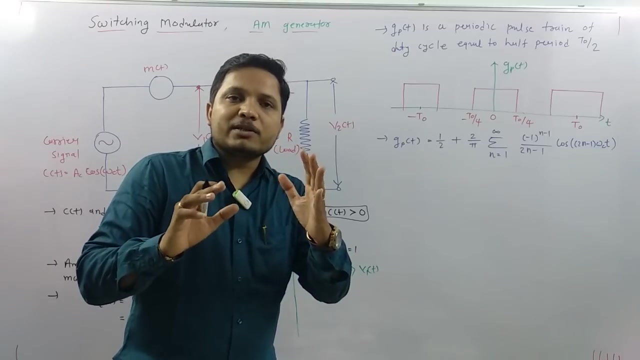 respect to some fixed period, this output is changing with some pulse train. With respect to fixed period, this output is getting change with fixed pulse train And that is purely based on V1T. Periodically it is changing with some pulse train, So V2T- this output. 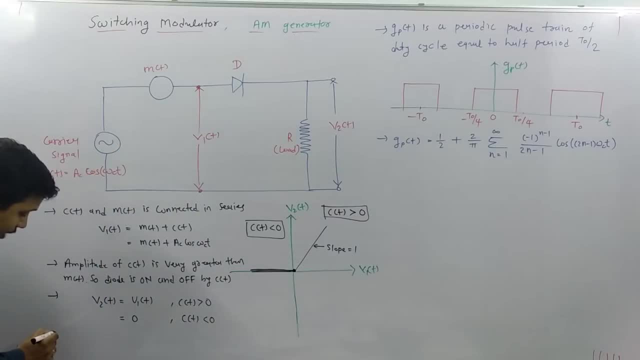 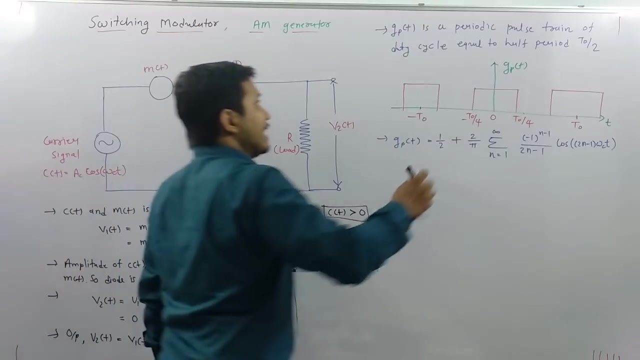 periodically So we can say: output V2t, that is continuously getting repeated periodically. So we can say it is V1t into, let us say, pulse strain is Gpt. So let us say, this pulse strain at which it is getting repeated, that is Gpt. Now see that Gpt, that is a periodic pulse. 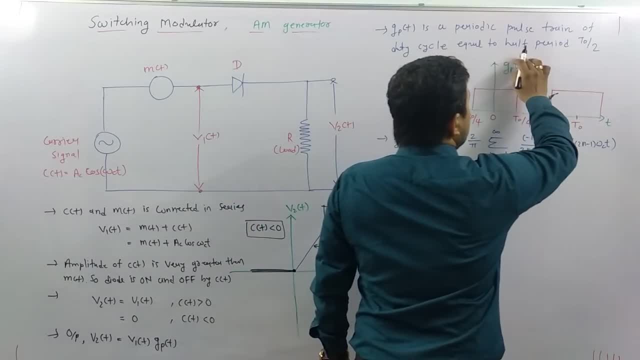 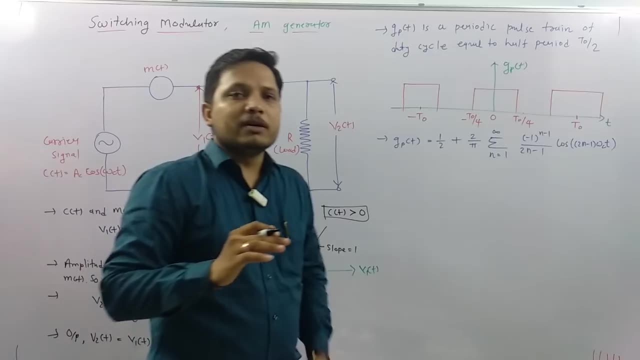 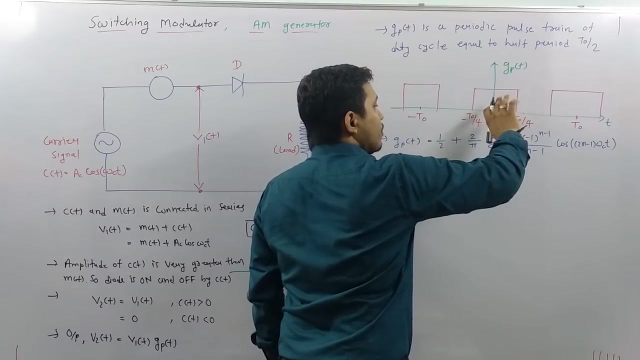 strain of duty cycle equals to half of the period. So its duty cycle is t0, its pulse strain, that is having width of t0 by 2. If I say at center its value is there, then t0 by 4 over this side and t0 by 4 over this side. 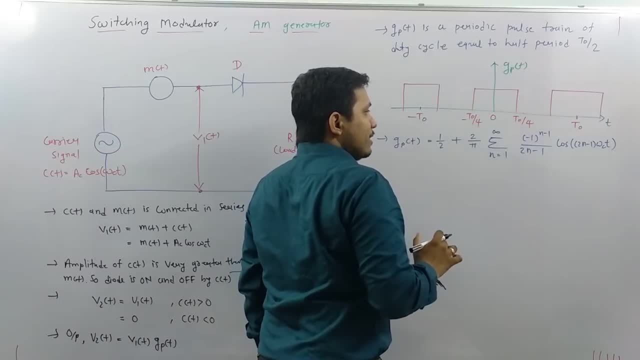 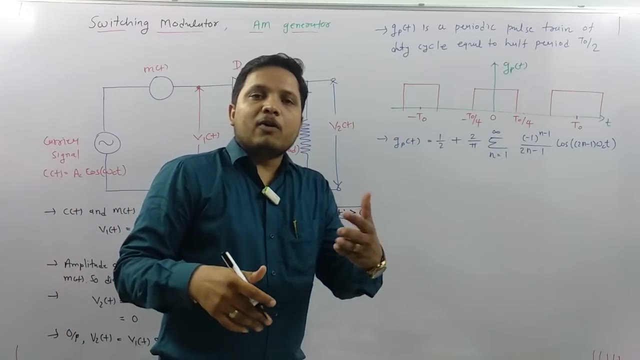 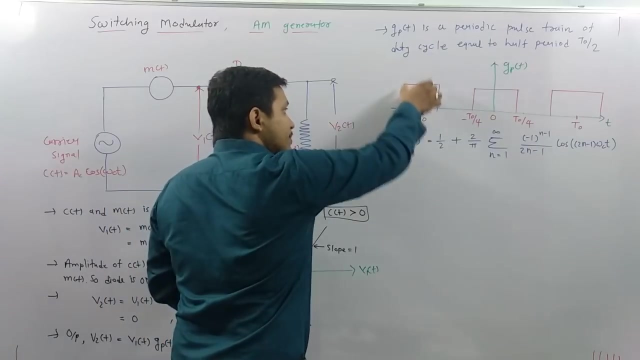 It will make its width to t0 by 2 and that is what keeps on repeating. So that is the pulse strain by which this output is periodically received at V2t side. So ultimately, for this amount of pulse period, V1t will get followed over here. For this period output will be: 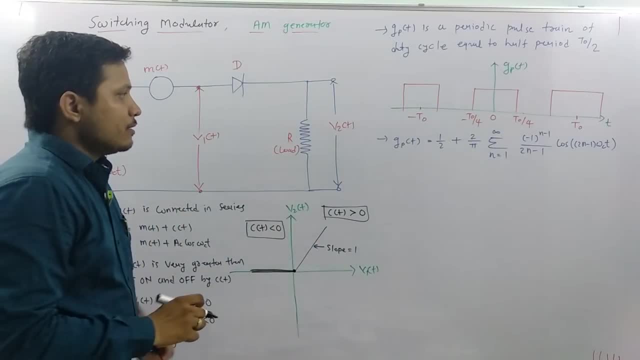 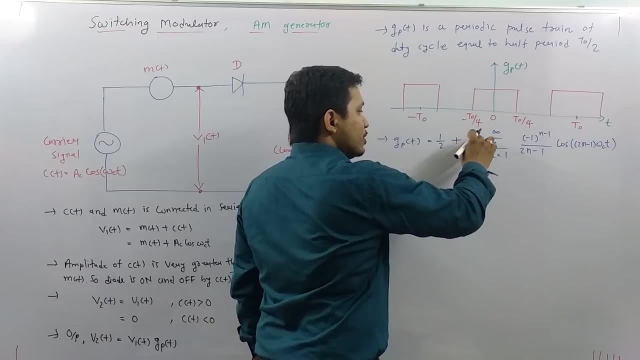 0. So that is what the basic meaning of it Now see, based on Fourier series, we can replace it. So that is what the basic meaning of it Now see, based on Fourier series, we can replace. isn't that GPT like this, That is, half plus 2 by pi summation, n varies from 1 to infinite. 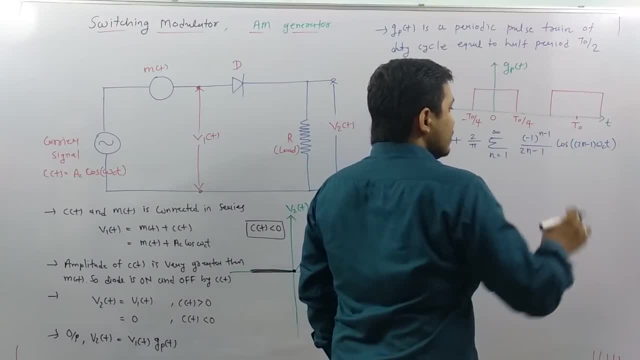 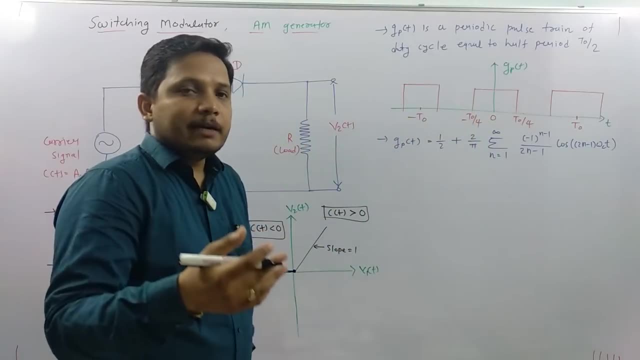 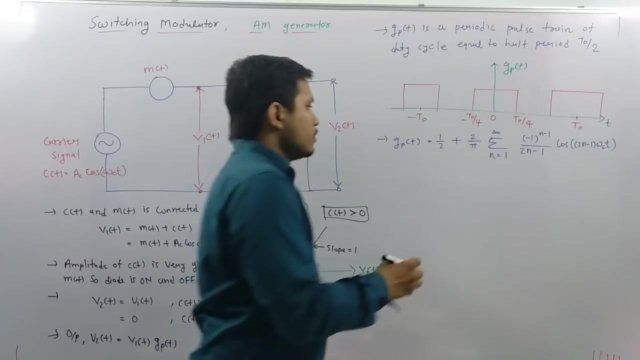 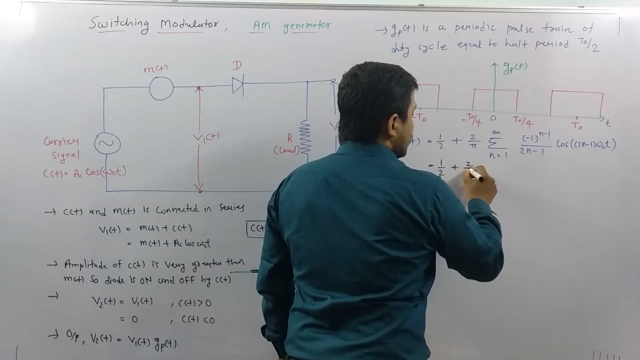 minus 1 raise to n minus 1, divided by 2n minus 1, into cos of 2n minus 1, omega cd. Now see, let us make it in terms of calculation frequency points. So if I re-evaluate this, in that case this will be half plus 2 by pi. if I place 1 over here in this, then this will be: 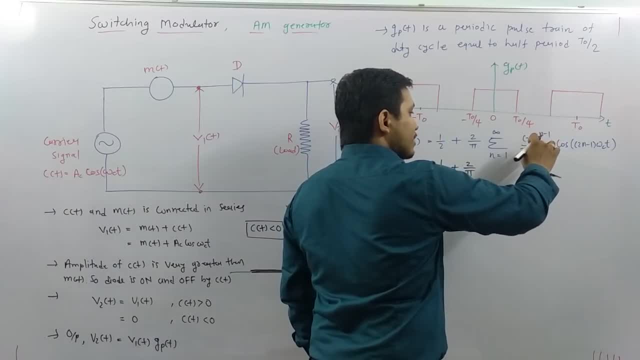 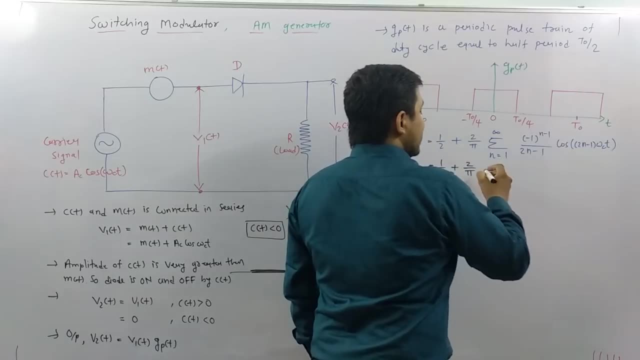 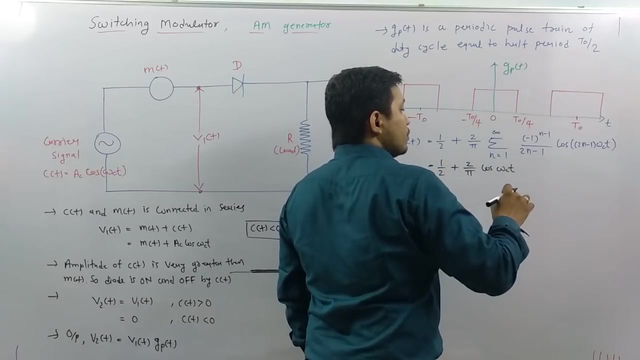 minus 1 raise to 0, so that is 1 divided by 2 minus 1, so that is even 1. into 2n minus 1, that is 1 omega cd. it means this will be cos omega cd. Now, if you place value n is equals to 2. 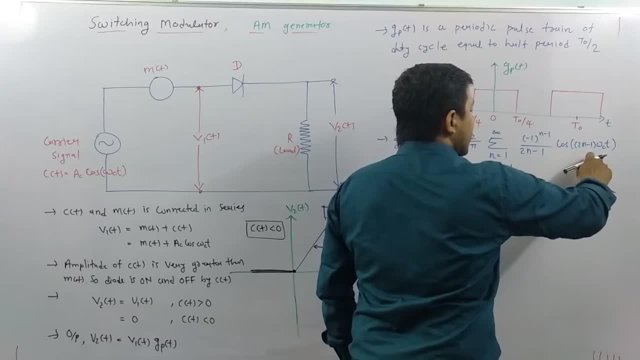 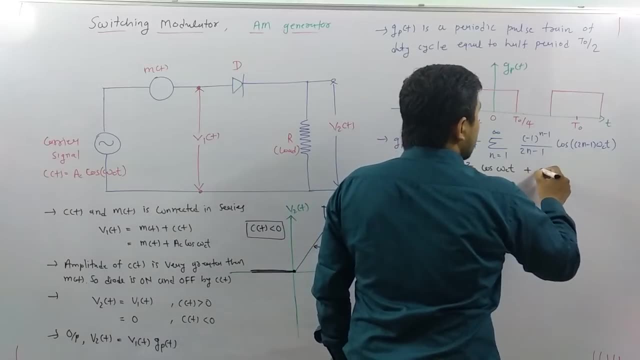 then there will be some term and this frequency component will be 1 over here. in this case this will be minus 1, raise to 0. so that is 1 divided by 2 minus 1, that will be 4 minus 1 means 3, so 3, omega cd. so there will be some odd harmonics. 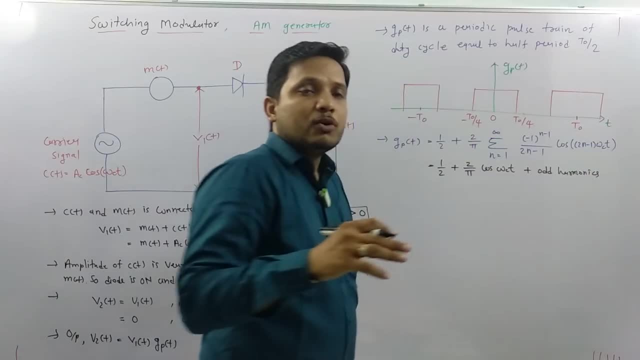 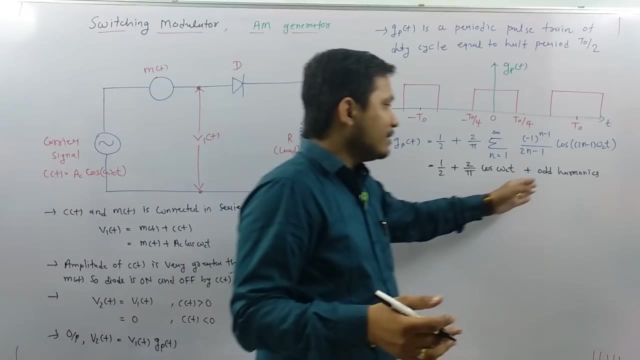 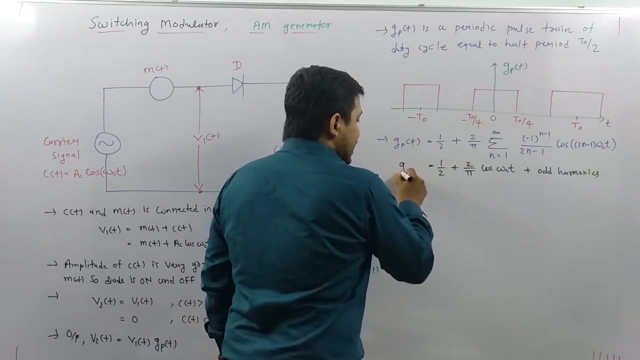 Now see, I am not writing odd harmonics. the reason is those harmonics are having higher frequency and we don't need to use that over here, so I am just neglecting this right now. the reason is: we don't need it right now, So now we have this GPT. 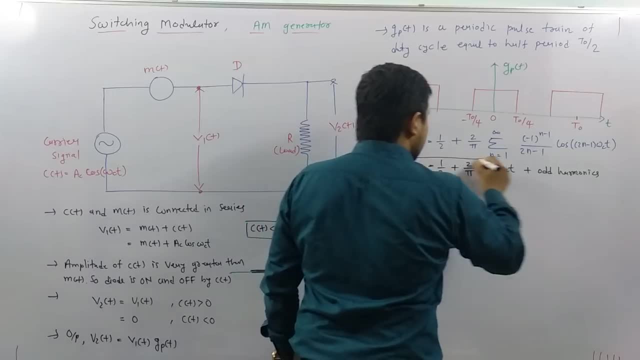 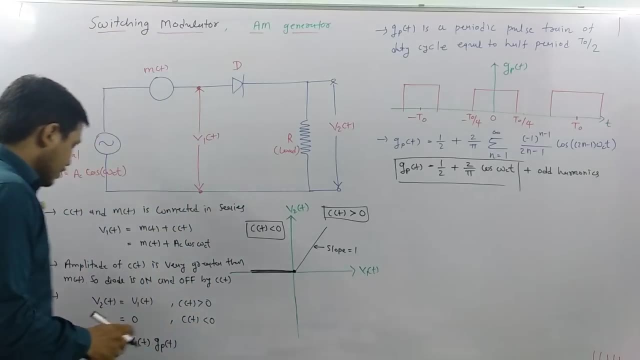 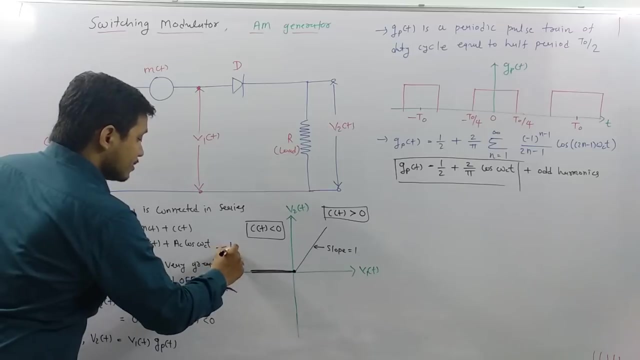 that is this and we usually neglect that odd harmonics. So now our output: V2t, now that that we can have it based on V1t, that is, mt, ac, cos, omega, ct into GPT. that is this. So if I say this is equation 1, this is equation 2, let us say this is equation. 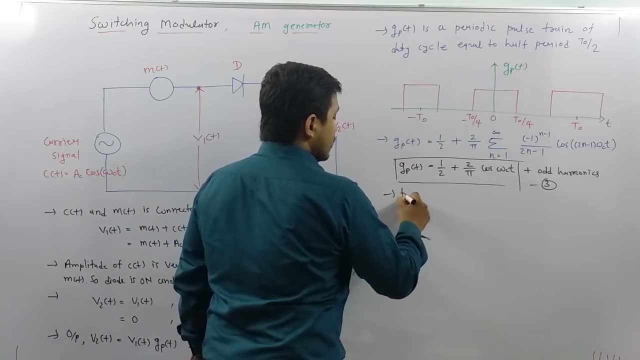 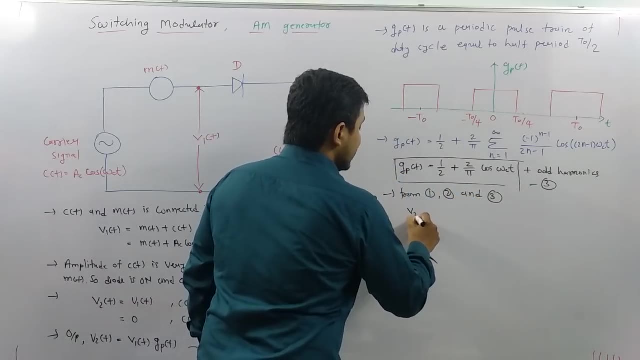 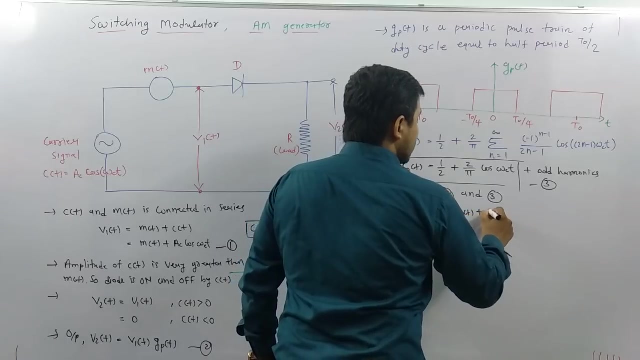 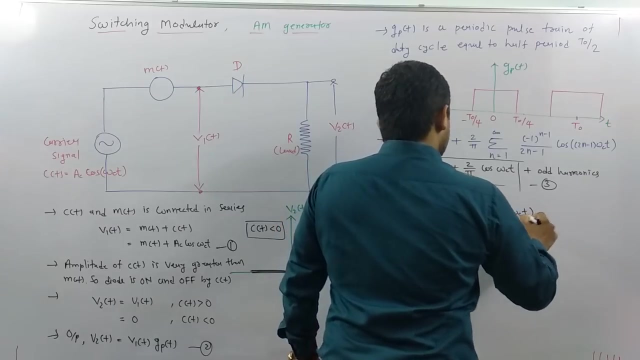 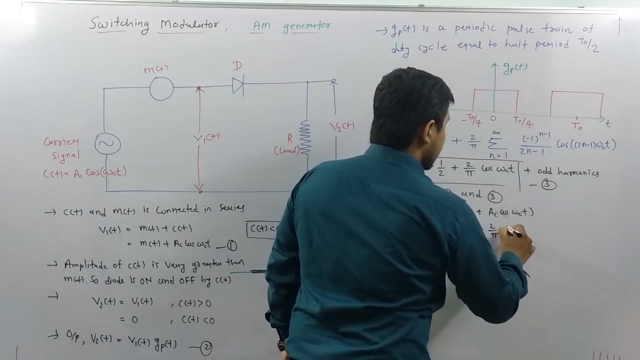 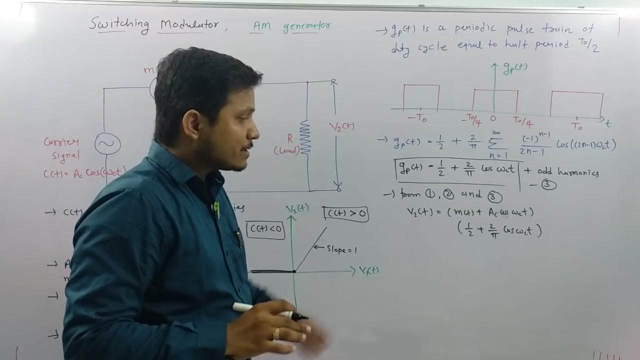 2. 3. so from equation 1, 2 and 3 we can say V2t, that is V1t, that is mt plus ac cos, omega ct, into GPT, that is half plus 2 by V2.. pi cos of omega ct and plus some odd harmonics will be there, plus some odd harmonics will be. 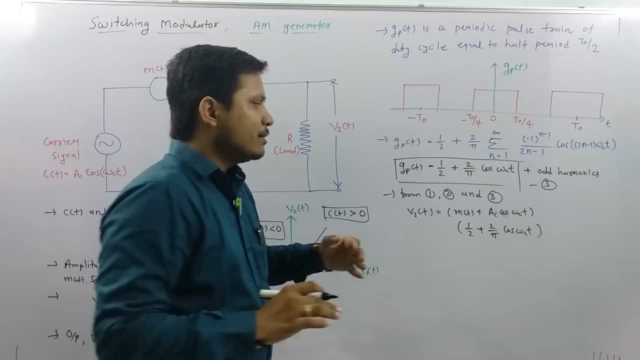 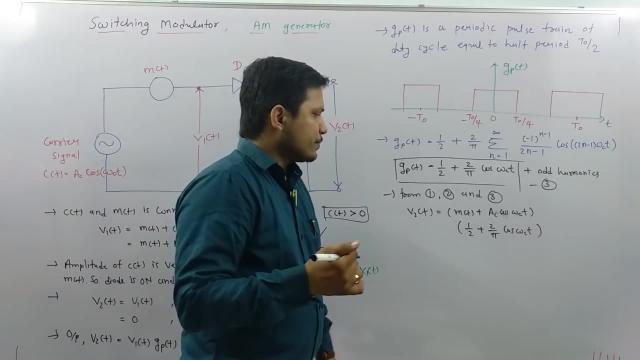 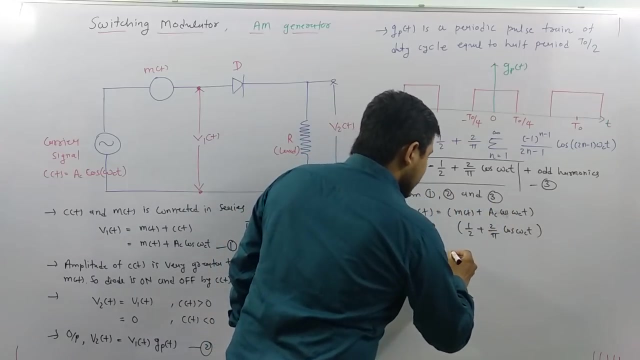 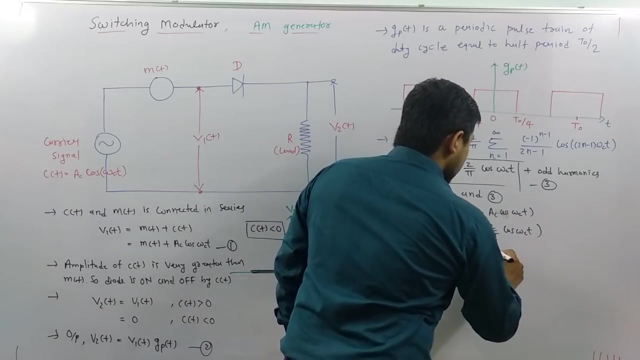 always there. so right now we are not writing it. neglect that, neglect those odd harmonics right now for simplicity of calculation. so now, if we re-elaborate this, then this will be: let us multiply this with half, so mt by 2 plus this is ac by 2, cos, omega, ct plus. 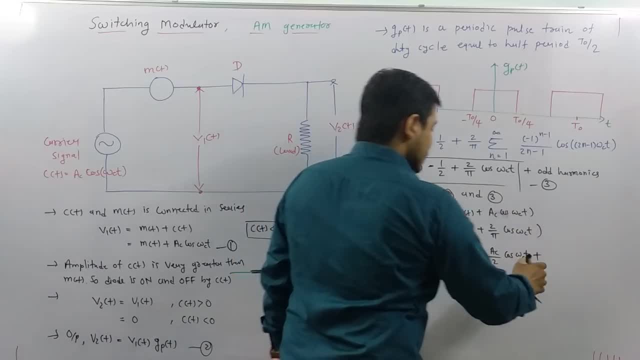 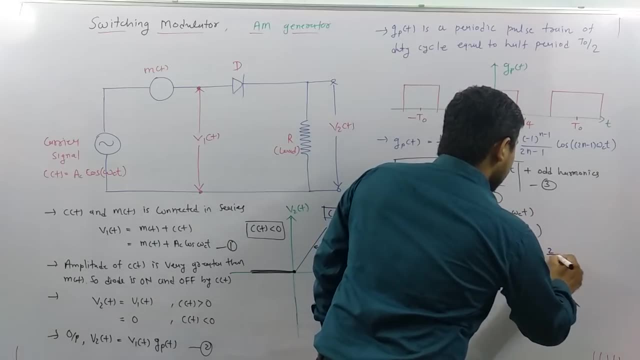 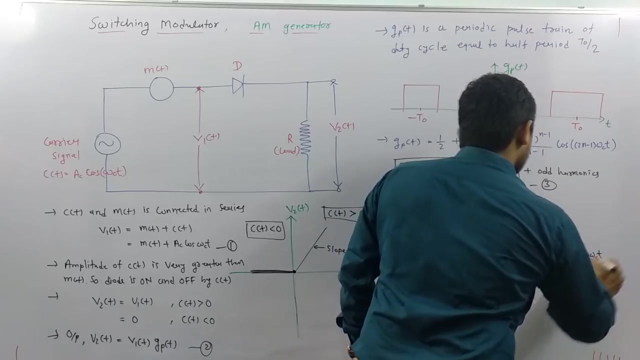 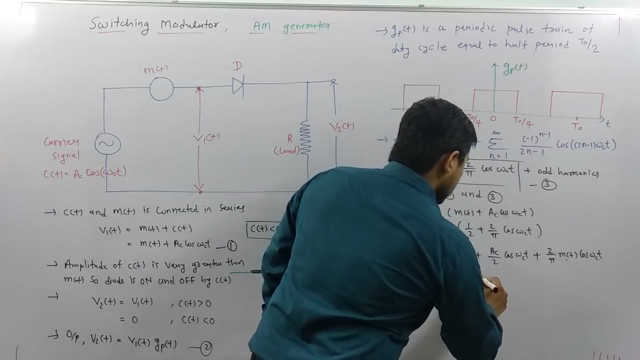 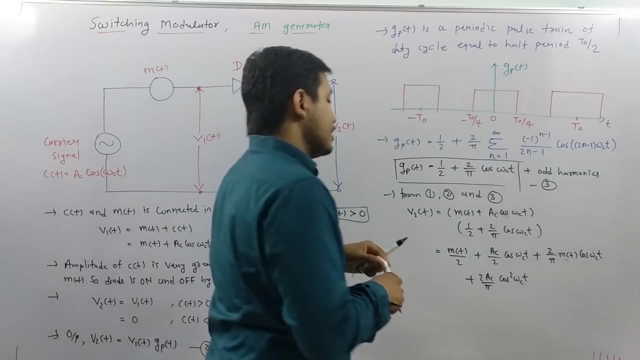 now multiply this term with this, so this will be mt- sorry- 2 by pi, mt cos omega ct plus 2 ac by pi into cos square omega ct. so that is what v2t now now see over here. if we see this equation, then this is modulating signal. this is: 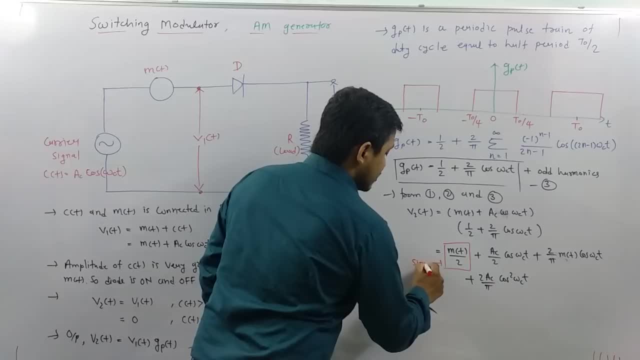 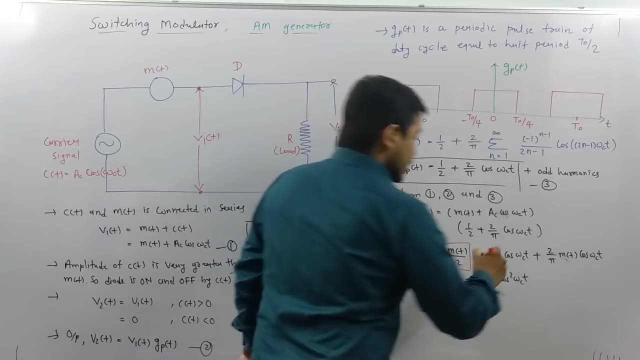 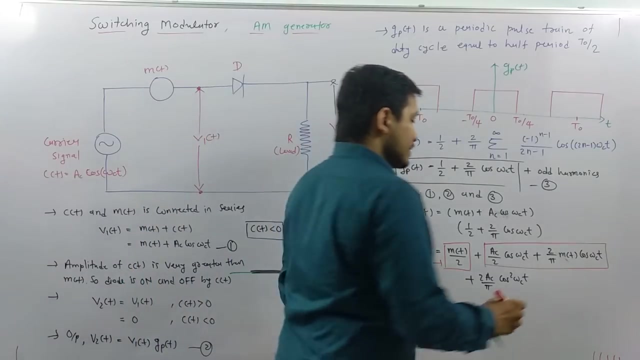 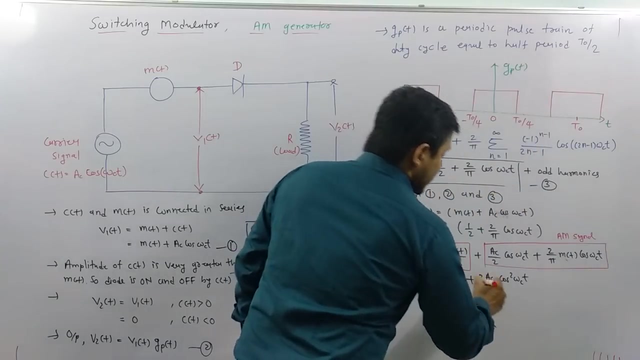 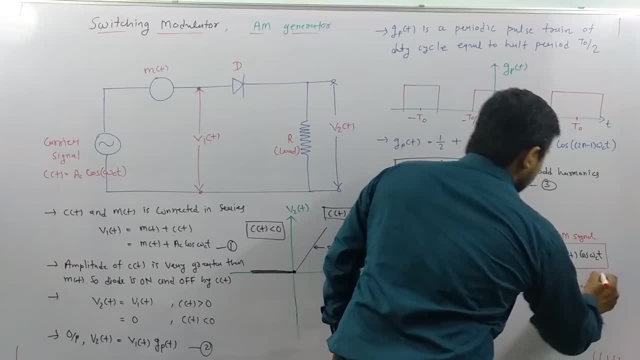 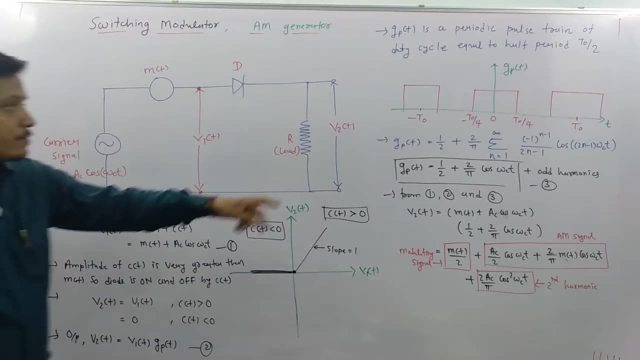 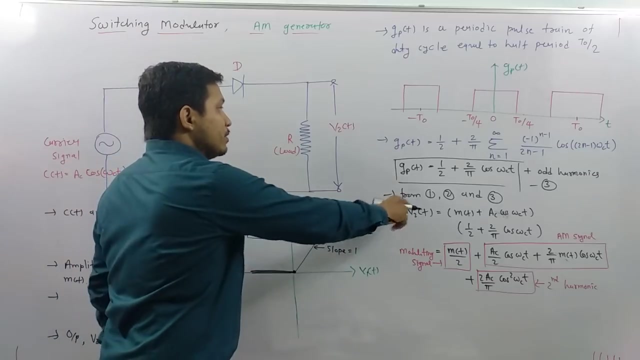 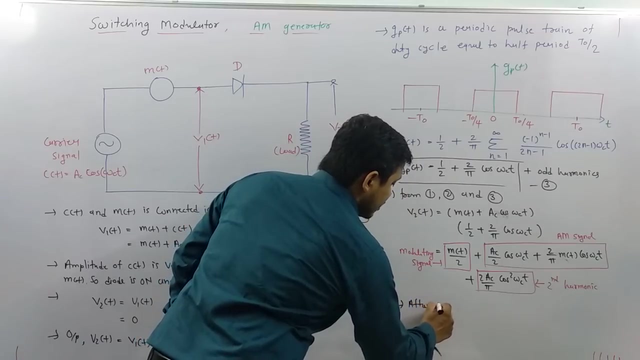 so this is second harmony. now, see, as i have told you, if you pass this v2t signal through bandpass filter, then you will be getting am signal. so if i pass this v2t signal through bandpass filter, then my output yt, after bandpass filter output yt. now that will be. 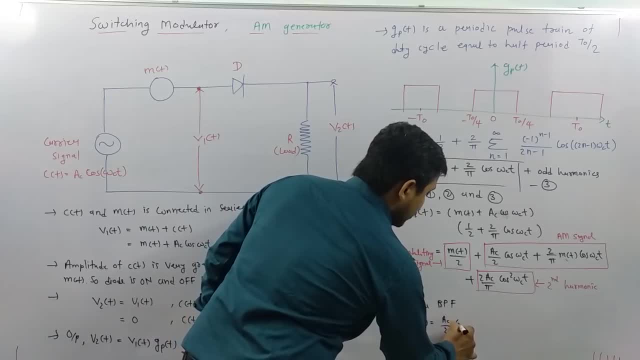 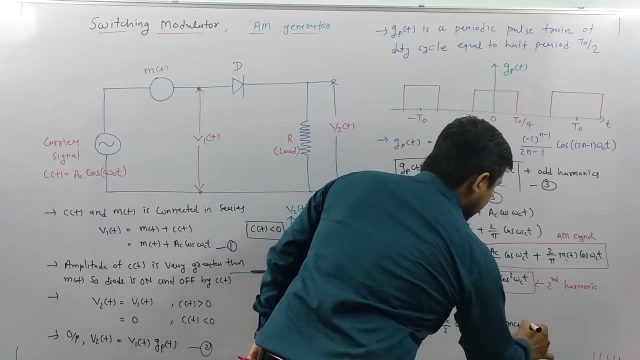 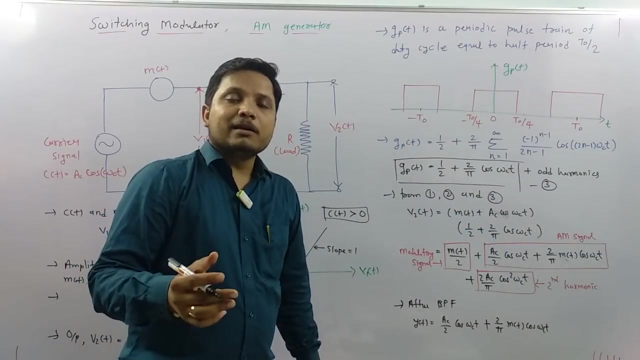 ac by 2 into cos of omega ct, plus 2 by pi mt cos omega ct. that will be my output. now see, i will represent this signal in terms of standard form, so it will be more clear. so, if i represent this in terms of standard form, 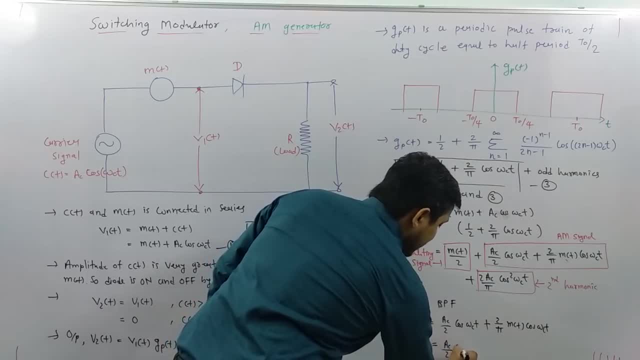 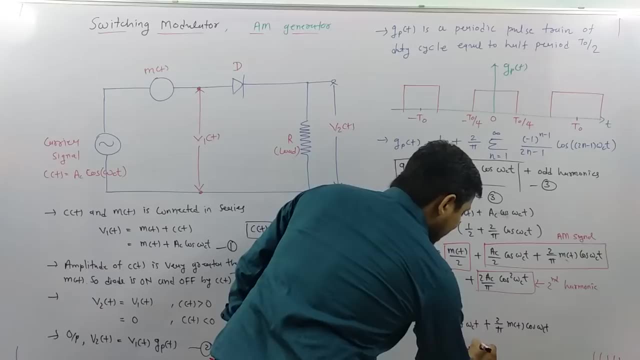 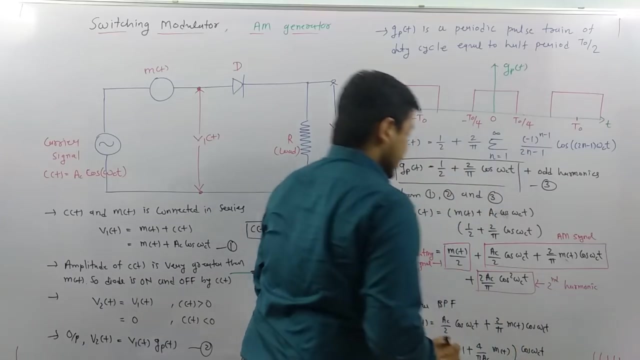 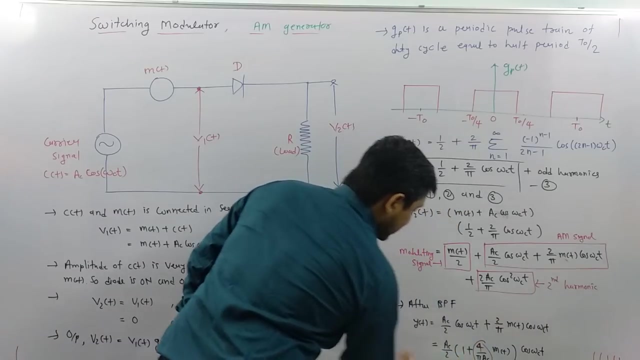 then it will be ac by 2 into 1 plus i'm taking ac by 2 cos omega ct common. so now this will be 4 by pi ac, 4 by pi ac mt into cos omega ct. so this is modulating decay, where this 4 by. 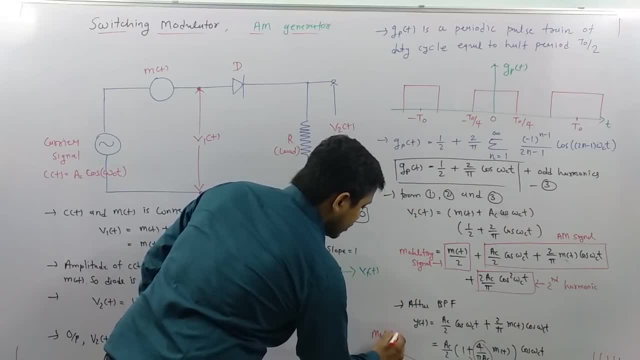 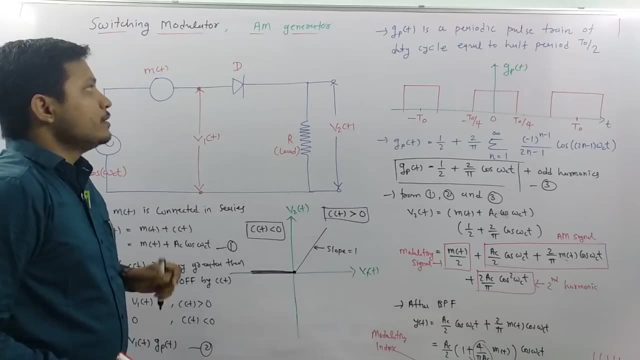 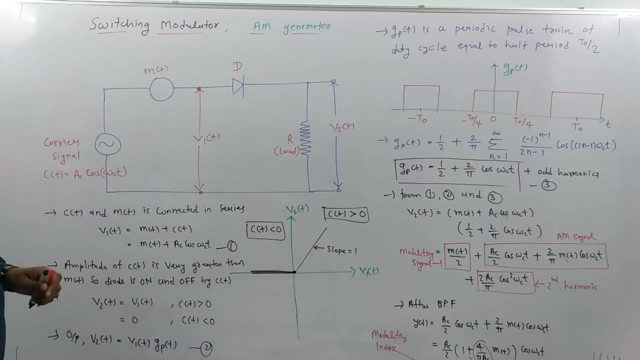 pi ac, that is modulating index of this am signal, which is what we are modulating, the switching modulator. so, ultimately, this is what switching modulator which is generating am signal and that knock-out and termination. we call this cancer. you, so you can you tell in. 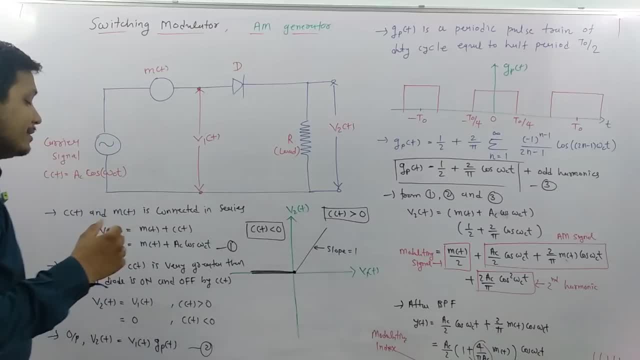 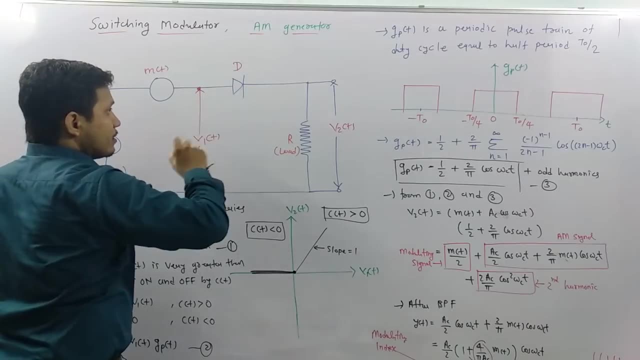 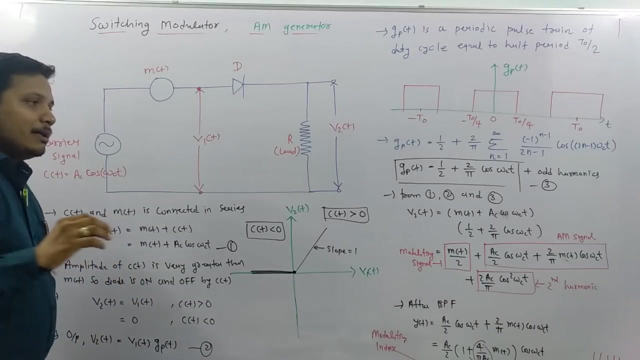 modulator which is generating a variation in就是 signal and thatье and that generation of am signal that is based on switching modulator, where switching element is this diode. so this diode is switching element and by that switching element we are generating am signal. let us have small brief about this so again it will be pretty clear to all like. 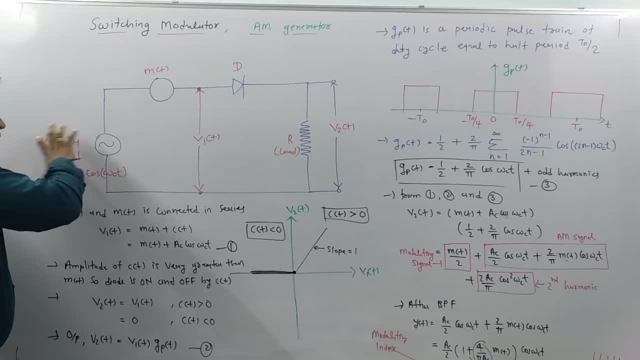 see how it is functioning, see here: carrier signal and modulating signal is in series. so here v1t, that will be ct plus mt. remember one thing: carrier signal amplitude is far greater than modulating signal. so this diode on and off operation, that will be justified by carrier. 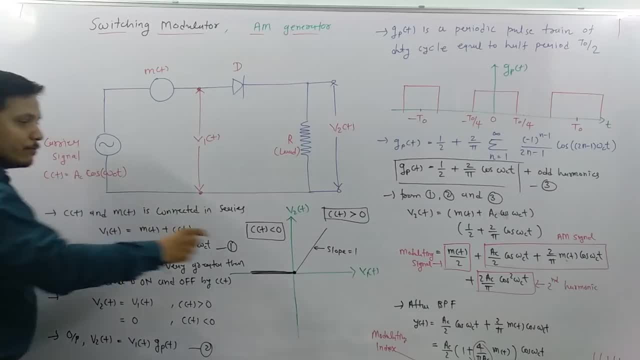 signal. so if carrier signal is positive, v2t is equals to v1t. if this carrier signal is negative, v2t will be zero. so v2t is periodically varying in between v1t and 0 and that periodic variation that we are justifying. 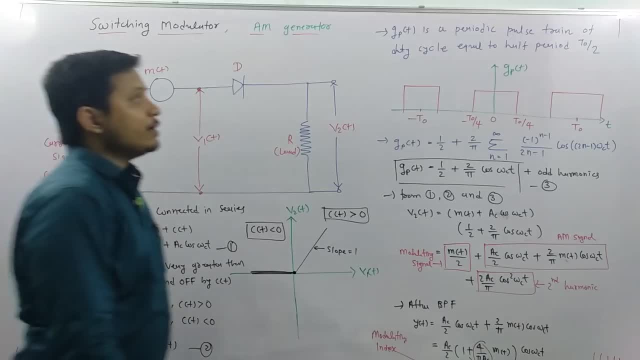 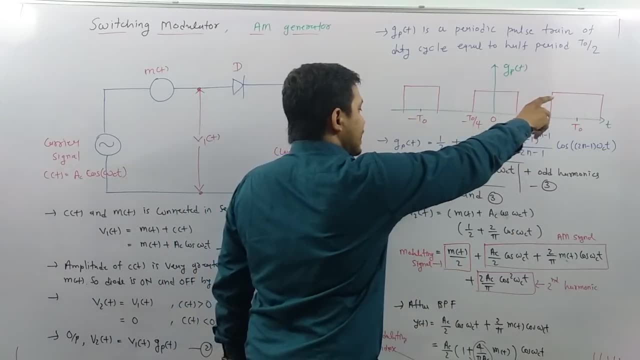 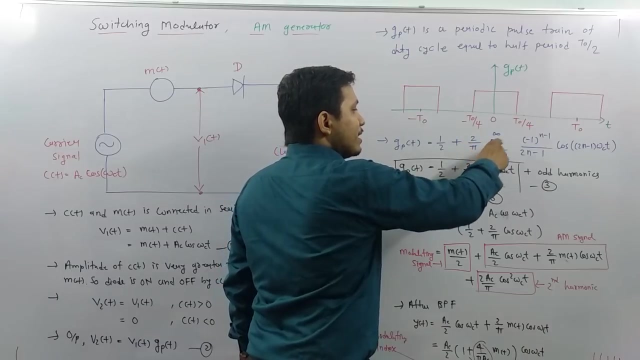 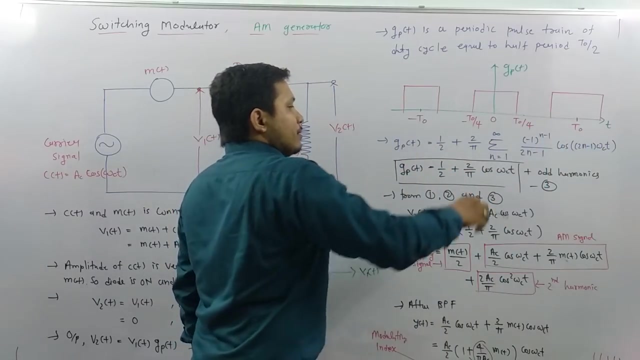 based on gpt and that periodic time period of duty cycle of t0 by 2, it is like this: and if you represent this gpt in terms of Fourier series, then that is gpt is equals to half plus 2 by pi. summation of n varies from 1 to infinite and this term where we are just placing few, 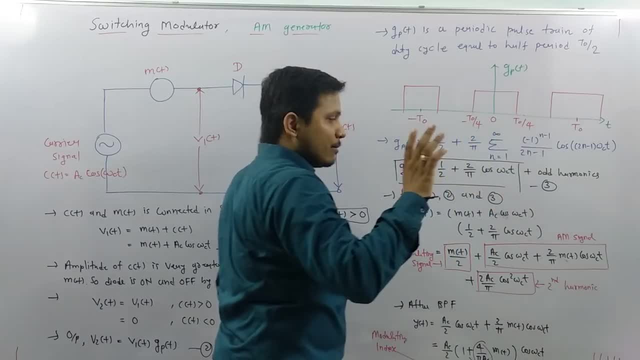 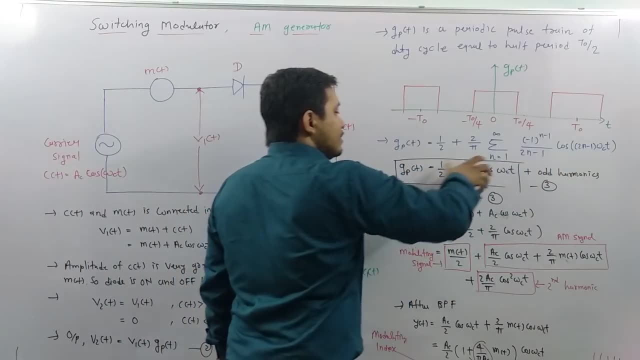 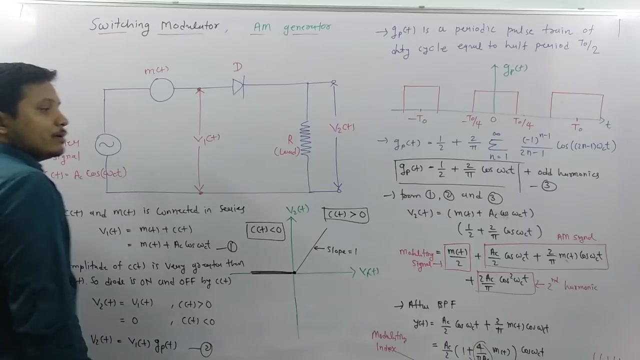 one harmonic only. we don't use odd harmonics here. the reason is that is having high frequencies. so I am just writing this equation to simplify that. and if we place this gpt v1t in v2t formula, then we will be having: v2t is equals to this. 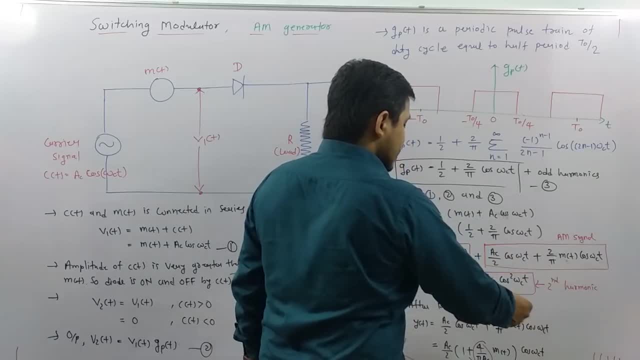 and if we place this gpt in v2t formula, then we will be having v2t is equals to this. and if we place this gpt in v2t formula, then we will be having v2t is equals to this. and that is, what combination of multiple signals where this signal, that is, modulating signal? 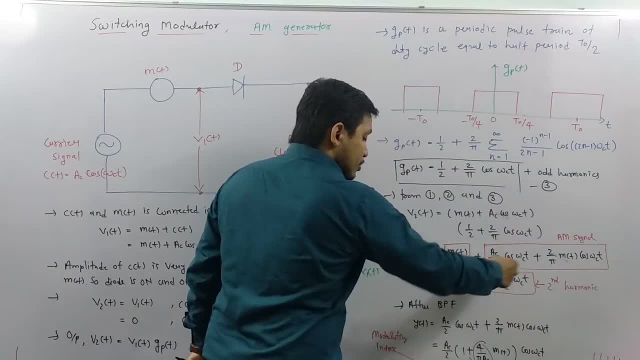 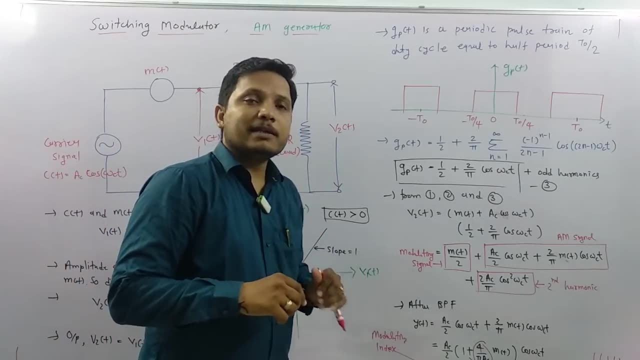 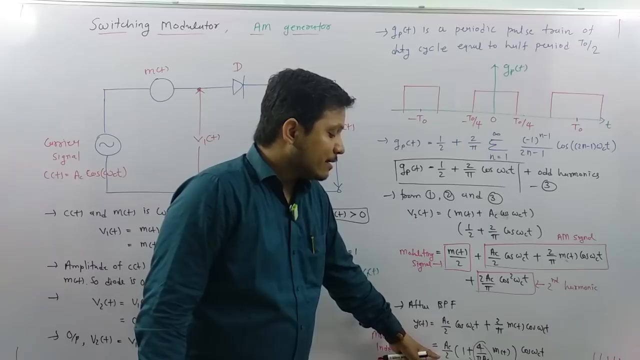 this is am signal and this is second harmonics. now, if you pass this signal through bandpass filter, you will be finding am signal. amplitude modulated signal. so this is what amplitude modulated signal and this is what I have represented in terms of standard form, which is having modulating index.